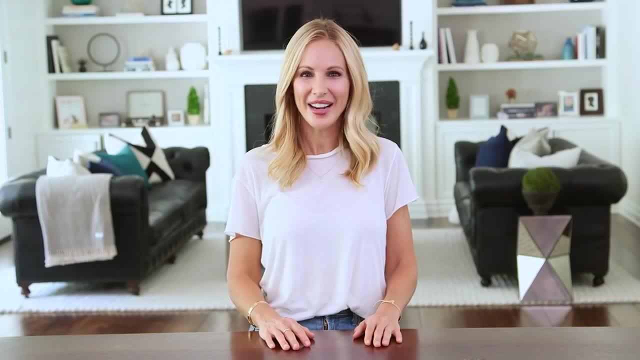 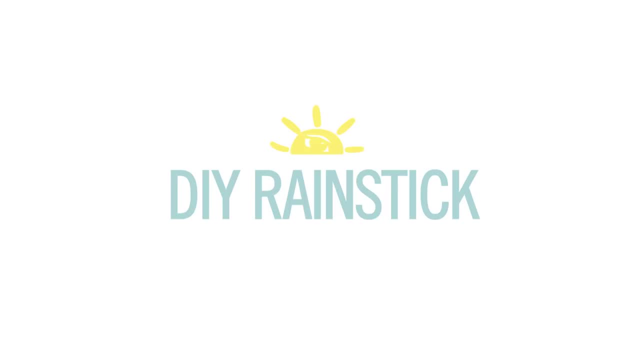 you how easy it is to make your own rain stick with just a few supplies you probably already have at home. I'm Brooke and I'm passionate about making beautiful things for my family on a budget. All you'll need to get started is an empty cardboard roll, some rice or bread. 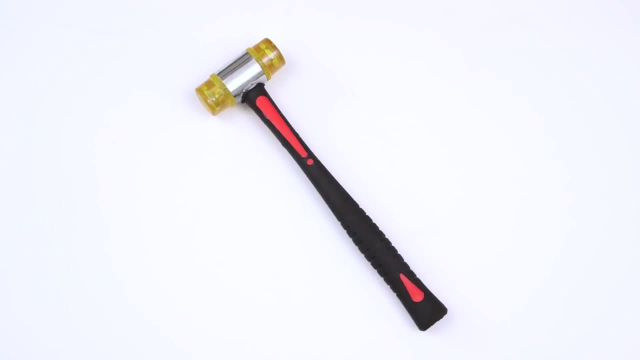 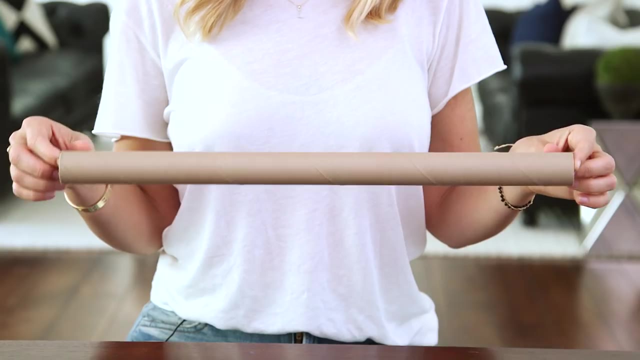 beans, small nails, clear packing tape and a hammer or mallet. We're going to start with our cardboard tube, which is going to be the body of our rain stick. I'm using one from an aluminum foil roll because it's a little bit thicker and more sturdy, but I'll show. 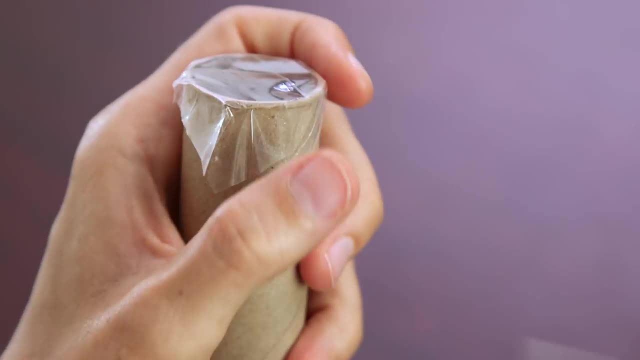 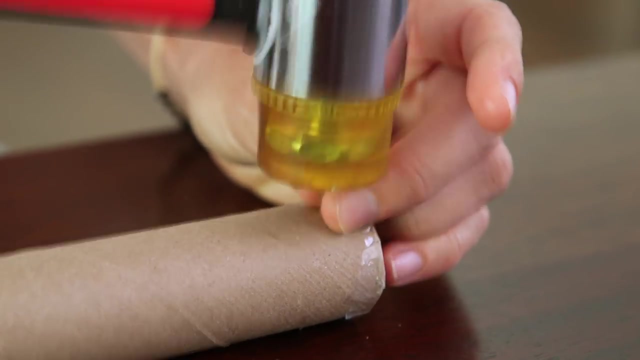 you another option later. if you only have a paper towel roll And the first thing you're going to do is tape off the bottom with some clear packing tape, Alright, our end is capped and now we're ready to start adding our nails. Place your first one near the end of the tube. 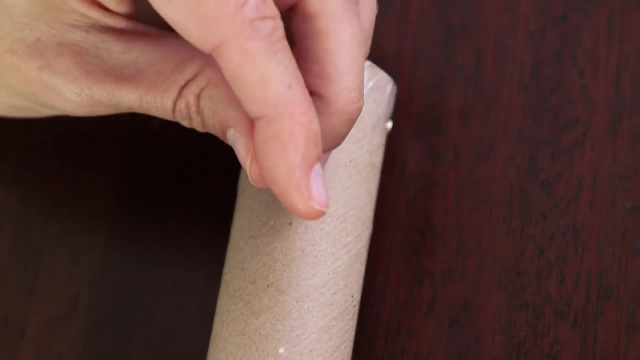 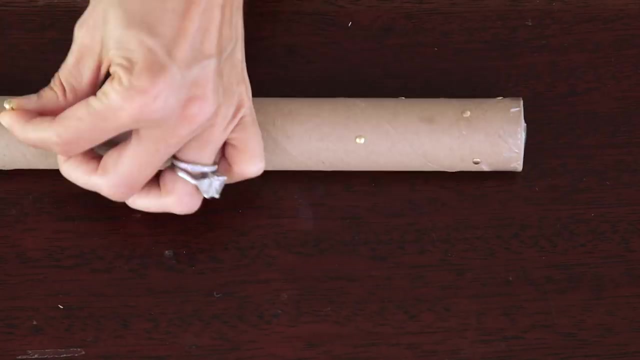 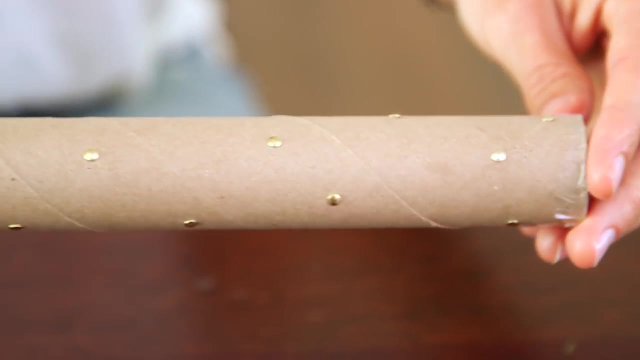 and hammer it in. Then rotate your stick a quarter of a turn, place your next nail a half an inch to an inch below the first one. Continue this process all the way down the length of your stick. Our nails are all in and it should look like this: My nails are really secure, but if you're 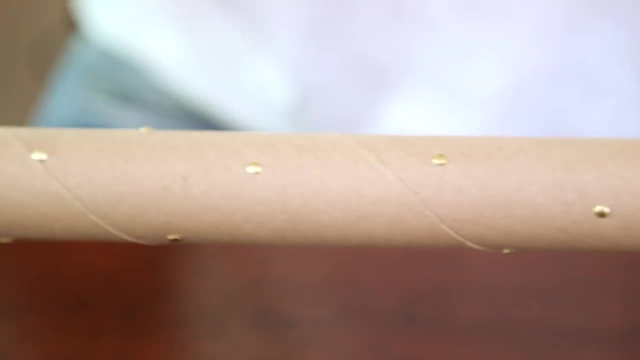 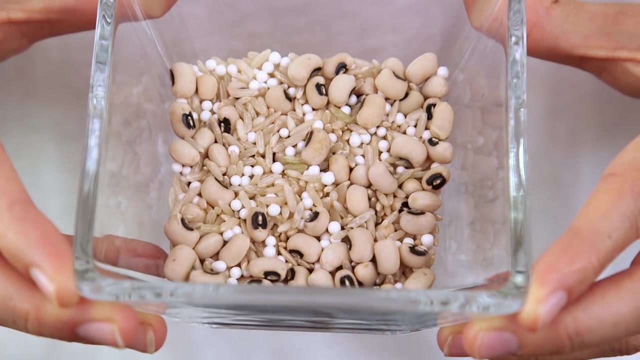 at all worried about little ones trying to take them out. you can cover the outside in duct tape or wrapping paper. Now for the fun part. we're ready to add our rain. I'm using a blend of black-eyed peas, brown rice and some leftover sprinkles. Then just take your. 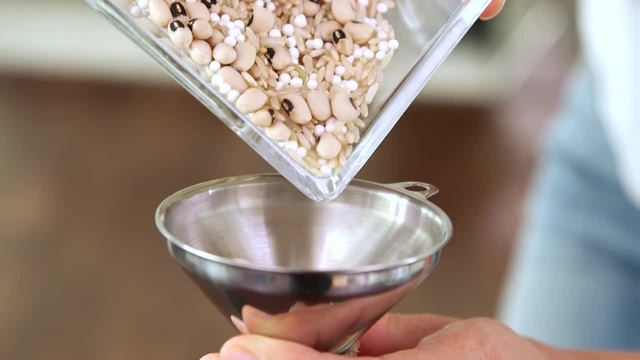 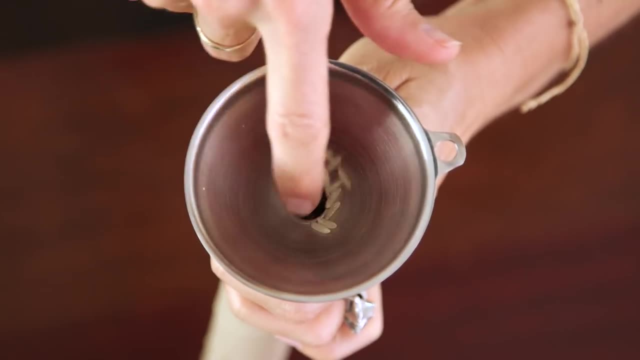 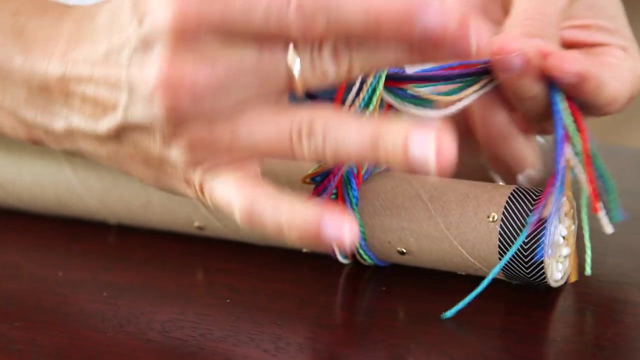 tube, add a funnel and let's make it rain. We're almost done. All we need to do is tape off our open end, and then I like to add a strip of washi tape at either end to create a clean edge and then tie on some embroidery. 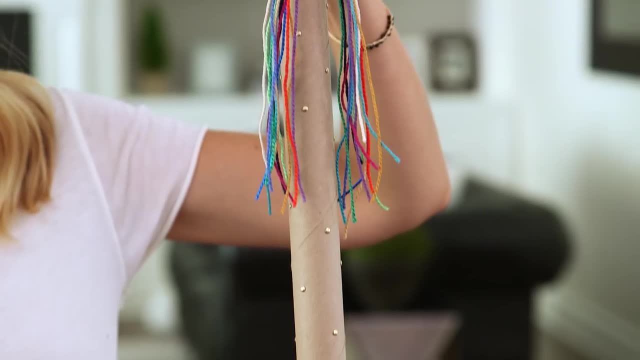 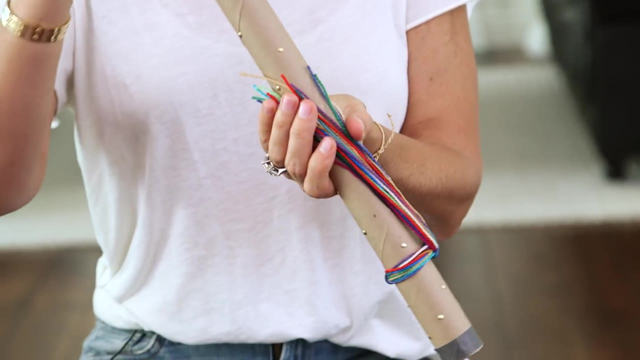 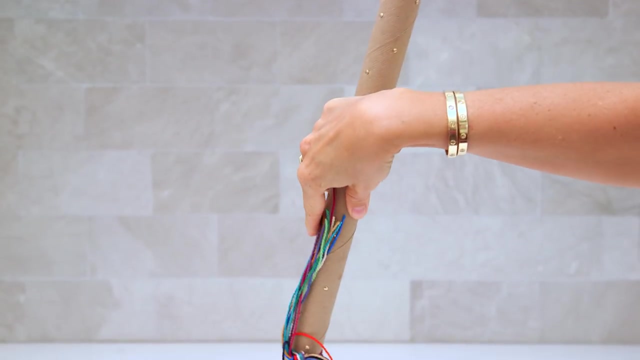 thread for a pop of color, Ta-da. I think this turned out adorable and the best part is it sounds just like a real rain stick. Let's test it out. These really sound incredible and they become kind of addictive to play with. We also made long ones with wrapping paper tubes that are great for older kids- Our favorite. 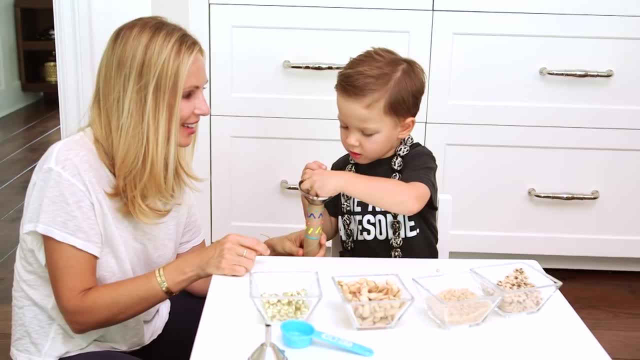 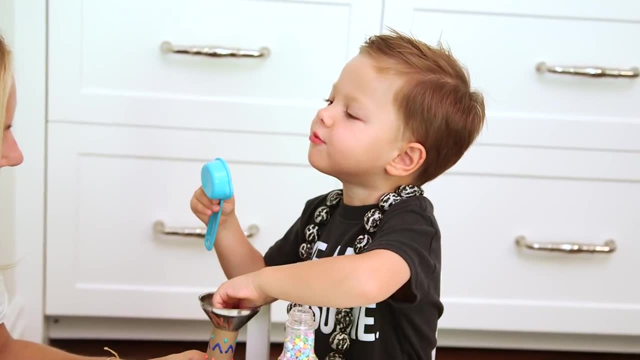 part was experimenting with a variety of objects to create different sounds. This turns it into an educational and fun play date activity. I'm making a rainbow sprinkles If you want to use a paper towel holder, and it's not strong enough to accommodate the.